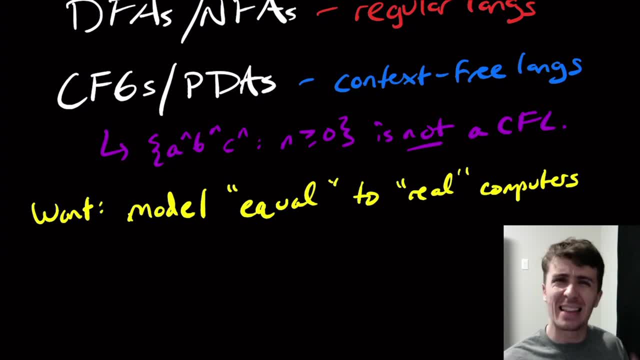 therefore our computers can't do so. it's kind of like the end of the line in some sense. so if we encounter something that's equivalent to our model and what we understand as computers that we used every day, then if we can't solve it in this model, then because it's equivalent to our 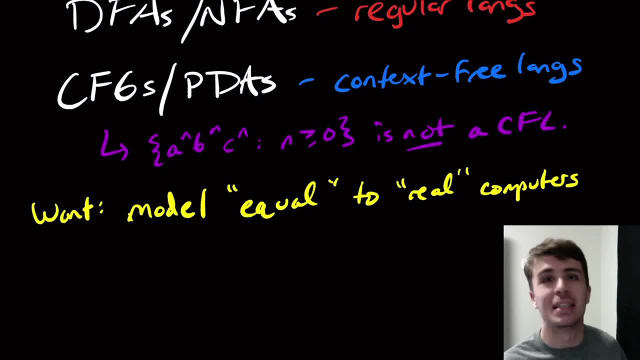 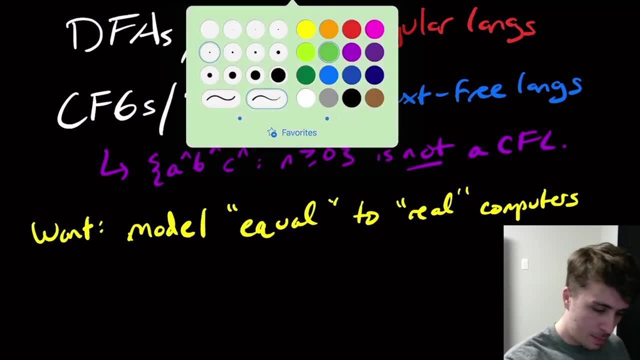 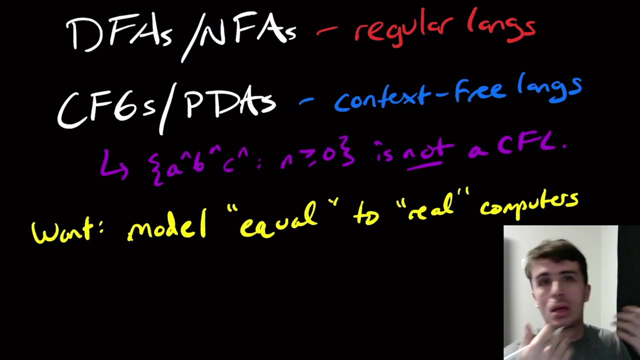 computers. we can't do it ourselves, there's no point investing into those, into trying to solve those problems, because they're impossible to solve. okay, so normally when I teach this in these class, in my classes, I would go into like the motivation in terms of how this came about, in like the history of it. but I'm 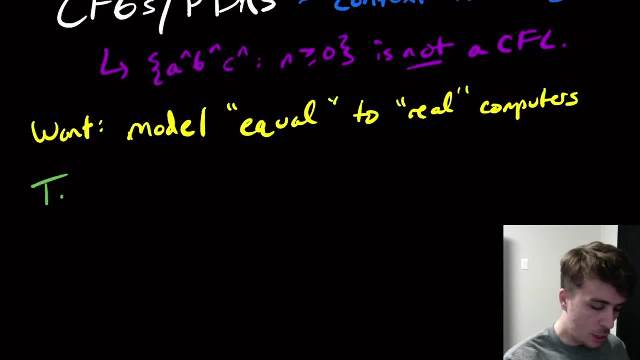 going to just skip right to the punchline and we're gonna talk about something called a Turing machine named after Alan Turing. and no, he did not name it himself. other people named it after him because he was so important to computing that I was terrible Turing machine. so what is a Turing machine? the? 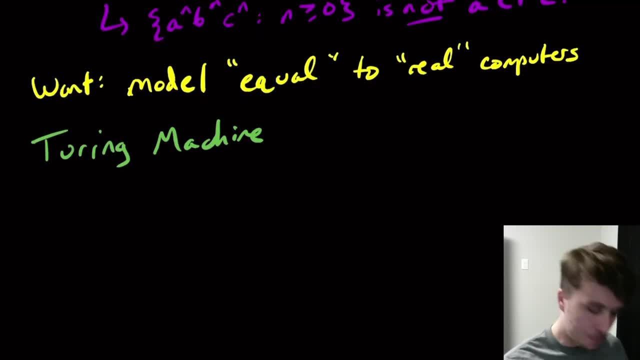 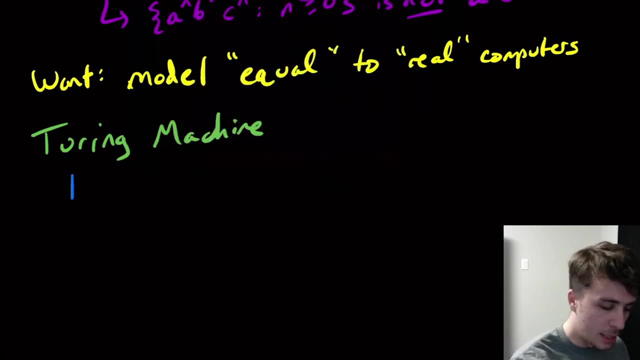 whole basic idea is try to generalize what a PDA can do. so the idea is that, instead of a tape- so we don't sorry- instead of a stack, so we don't have a stack anymore- instead we have a tape. and the way that this works is that we have a tape that looks like this: 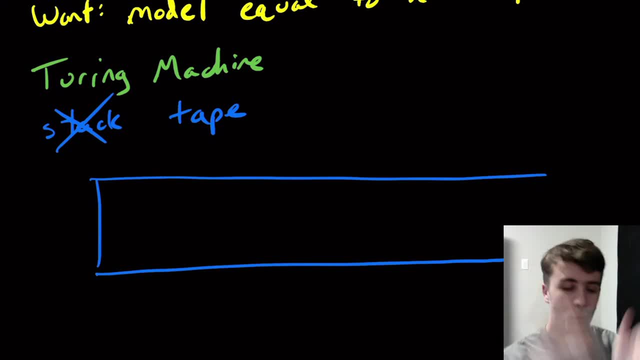 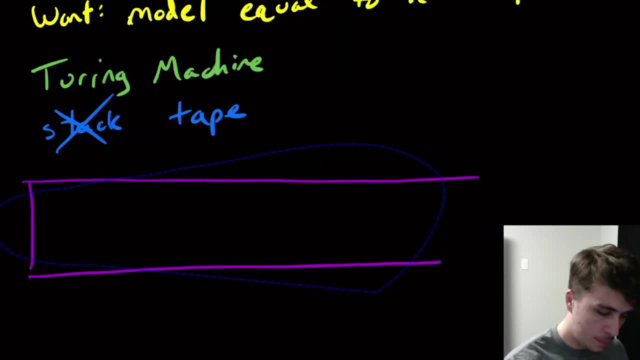 so it kind of looks like a stack that we rotated on the side and in some sense it kind of is a stack. let me change this to purple- and in each one of the on this tape we have a bunch of cells just like a stack, no different than a stack, and 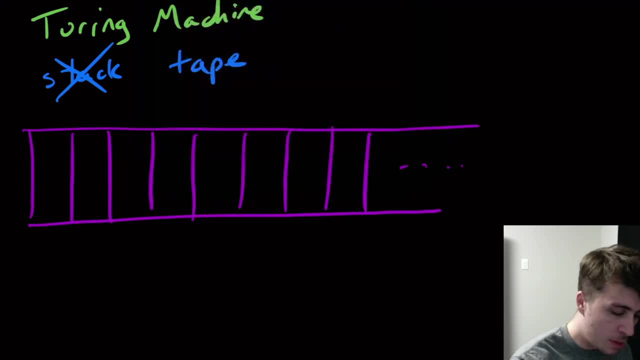 what we're going to do is we're going to put the input on the tape. so let's say that we have input W1 through WN, like this. so W1 through WN is the input here, and in order to investigate what is happening on the tape and what the the input is, we have something called a tape head. so 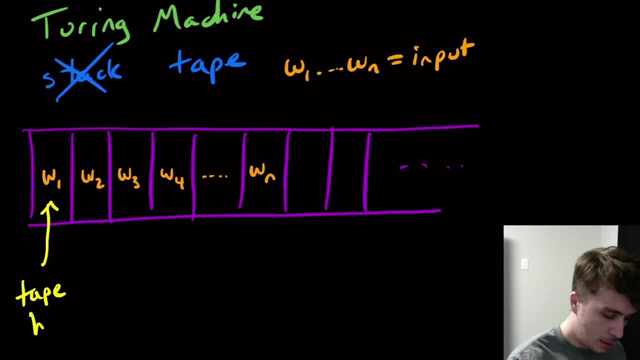 this is something called the tape head, and what it's able to do is it's able to move left and right, either backward or forward, one position at a time, as well as read the contents of the cell, and as well as change the contents of a cell. okay, so it's able to see. look at this. 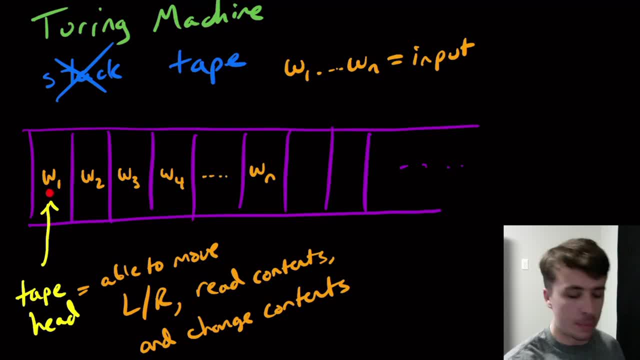 W1 right here and see: okay, yeah, it is a W1 right here, then maybe I'm gonna say I'm gonna move right and so after whatever's going to happen next, it's gonna, the tape head is going to point at this cell right here and we can say: oh, we're gonna change that W1 into an A for. 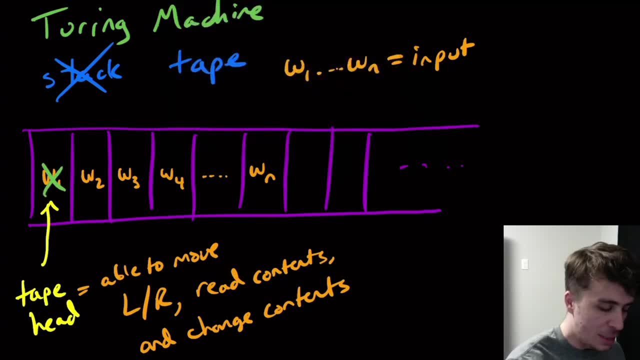 example. and so what would happen is is that I change this to be an A and then this cell is permanently going to change. oh sorry, not permanently. it's going to permanently change until I come back and hit the now button. so if I go to the next cell and I change it here- oh sorry, not permanently, it's going to. 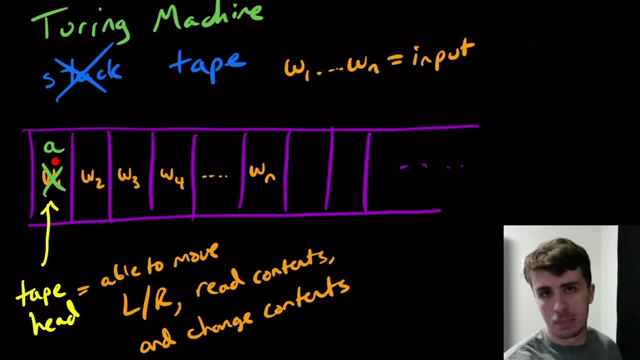 permanently change until I come back and and change it possibly at some later point. And so it's not like a DFA where we can only move right and we so. therefore we can't go back. but even if we could go back, we couldn't change the contents of the cell. So with a Turing 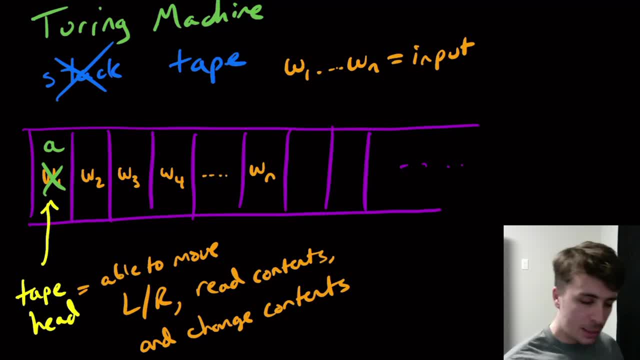 machine you're allowed to change the contents of the cell. And what happens if we are positioned right here, at the very last cell of the input, and maybe we change it or not, it doesn't matter What. if we decide to move right here, Then 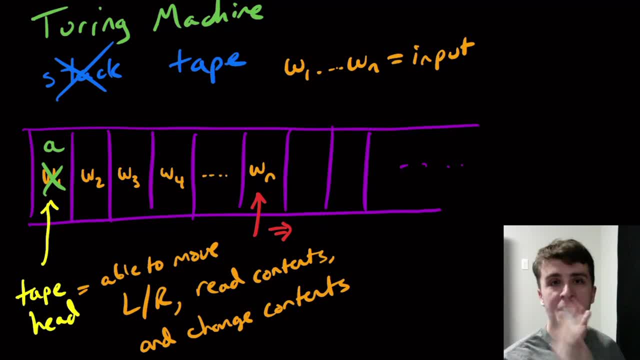 what will happen is, anytime we try to move right past the end of the input, then we're going to get some new memory and what is going to be placed? there is something called a blank cell. So, and this will be permanently attached to the, to whatever we have so far, anytime we encounter it or or create it. So 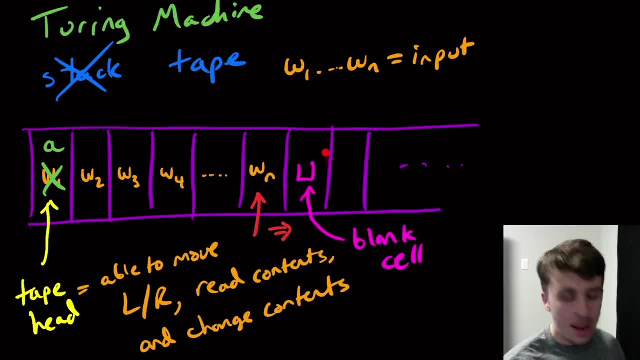 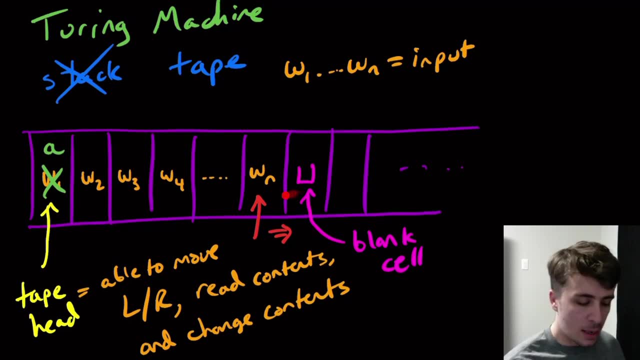 let's just say I'm right here and I move right, then this cell is going to forever be in our picture. We're always going to see this cell at some point in in what we have of the tape, And the reason why that's important is that this: 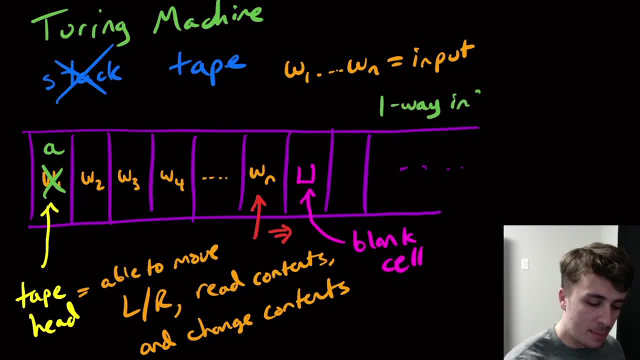 tape is one way, infinite, So infinitely, it can go infinitely far that way. So at every single point we're only going to see a finite slice of the tape. But the key is that we can have this grow as much as we want. We can make this tape. 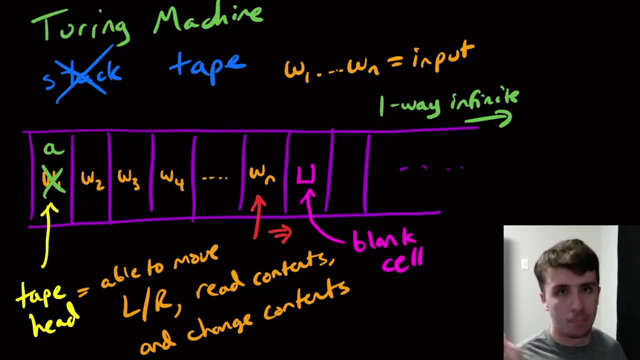 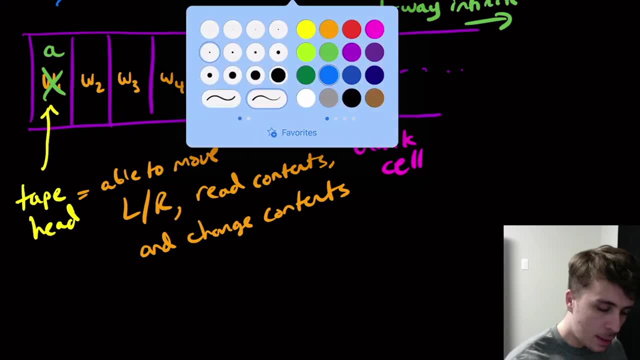 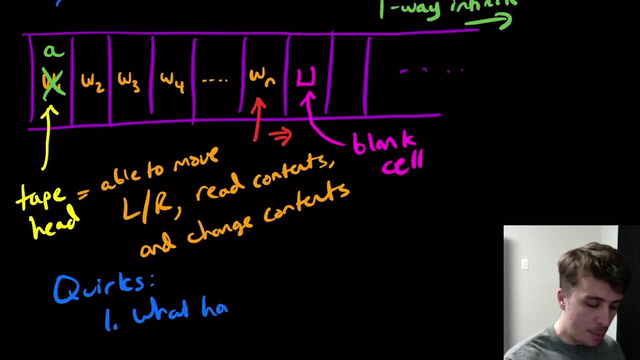 we can just keep going right as much as we want and potentially never stop at that point. Okay, so some quirks here that you may be asking What happens? I'll just write it: what happens if we move left off the first cell in the tape? So if we're in this cell over here and we decide? 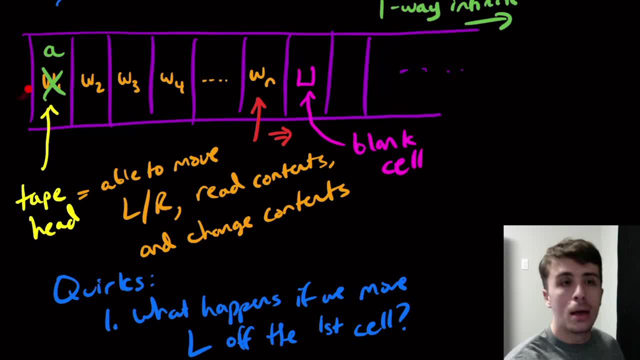 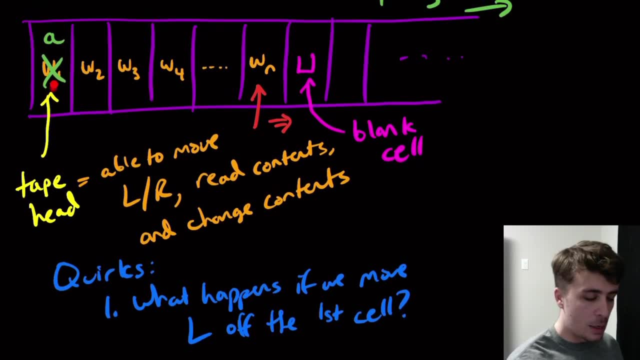 to move left, since it's only one way. what actually happens? So there are two philosophies here. Either you can just say you just stay in this cell, you don't actually move left, or you can say that the computation actually stops. 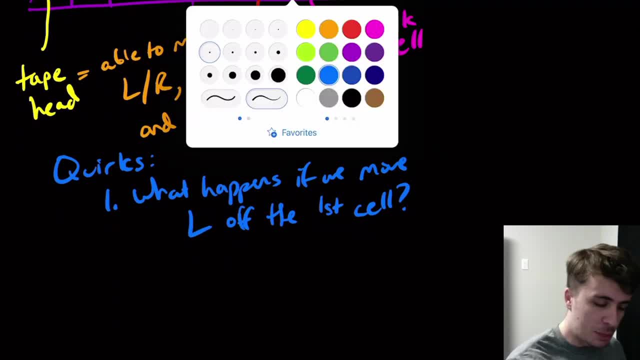 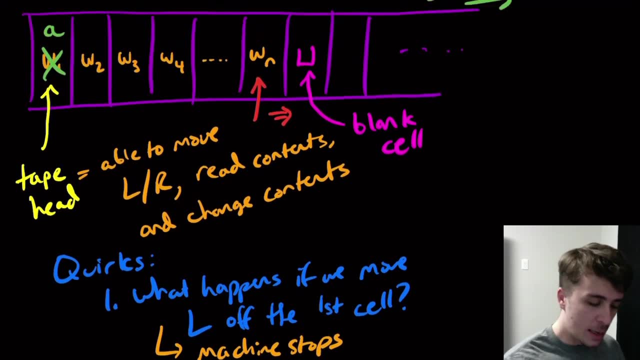 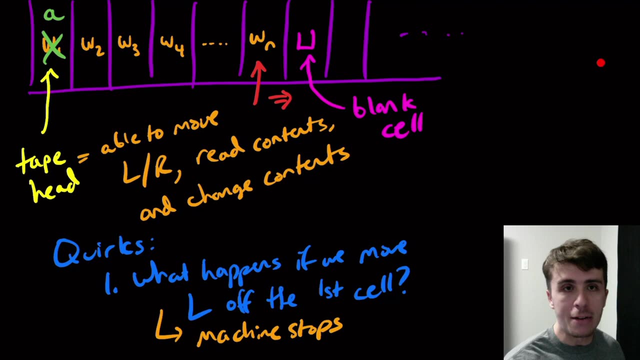 The machine stops, And so the perspective we'll take here is that the machine stops. Okay, so that's just a simple quirk that might happen. Another quirk that might happen is: could we potentially just keep going right forever? And the answer to that is yes, So can. 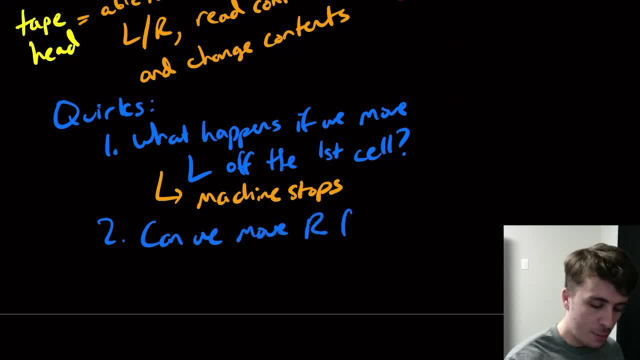 we move right forever, And the answer in this case is going to be yes. So I'm not going to restrict you, just to keep moving right. You could reason that the machine doesn't really do anything at that point and we're going to have 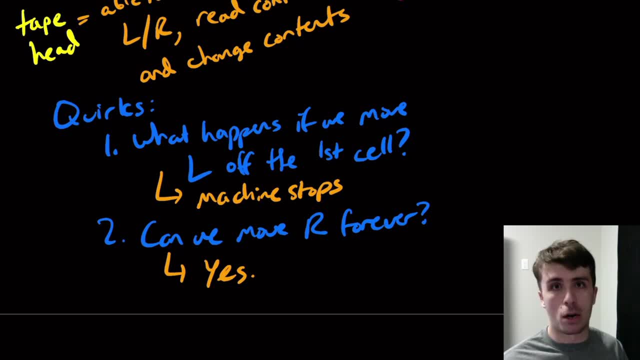 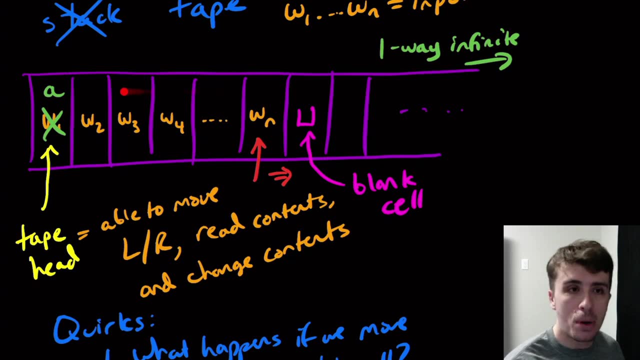 to take a look at that when we define the model precisely. But that's essentially what a Turing machine is: a one-way infinite tape where you present the input adjusted at the beginning of the tape, right here, And if you try to go off the left then the computation stops. The terminology there is, quote unquote. 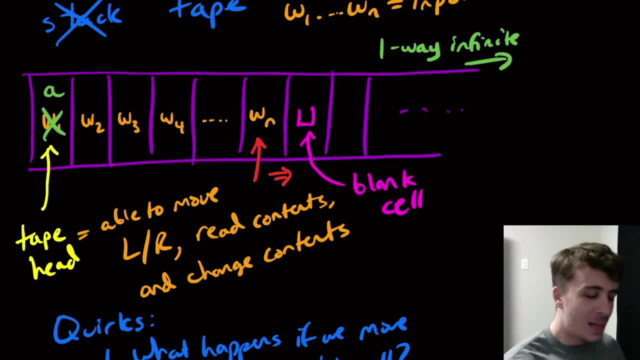 hanging yourself, but that's not a really nice term. So the computation stops. You can move left and right one cell at a time, every single transition. You can change a cell to be any value that you want, as long as you specify what things can be stored there in. 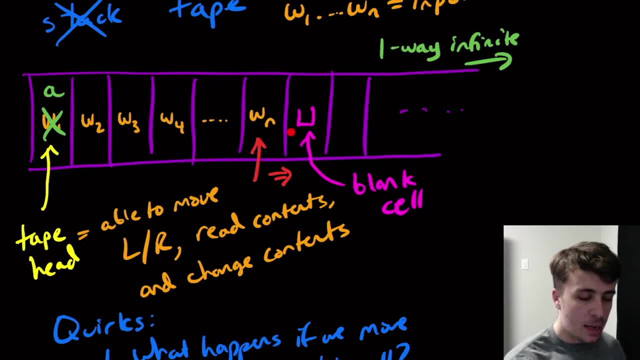 the first place, and if you try to move right past the furthest thing that you've ever seen, then you're going to acquire a new blank cell, And this cell operates just like any other cell here. You can change it to be anything. In fact, you can change any of these over here to be blank cells also. 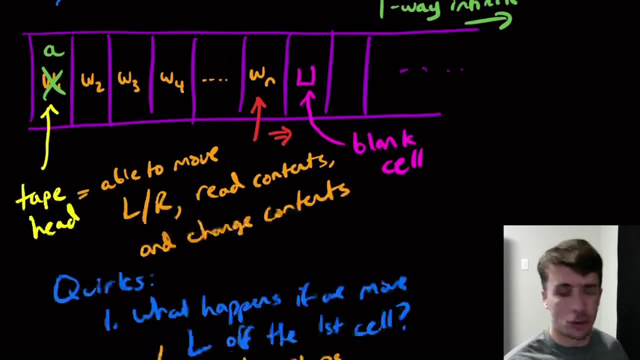 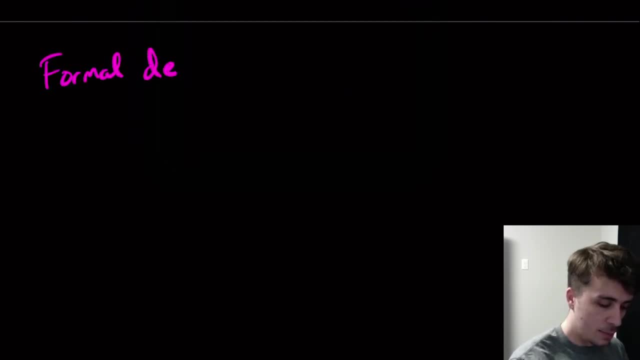 You don't have to keep these non-blank or whatever, All right. so let's look at a more formal definition of a Turing machine. So it's a state-based machine, just like the DFA's and PDA's were. So Q is a finite set of states. Okay, we have an input alphabet, just like before. So this: 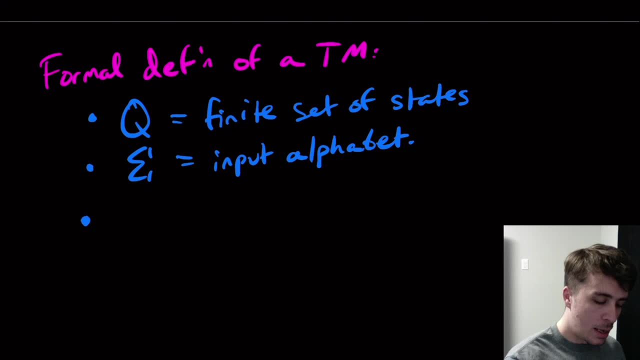 guy is also finite. no difference. there We have a set of all things that are belonging on the tape, So I didn't actually use this for PDA's, but it's kind of important. here We have a set, gamma, which is the tape alphabet, So it's the 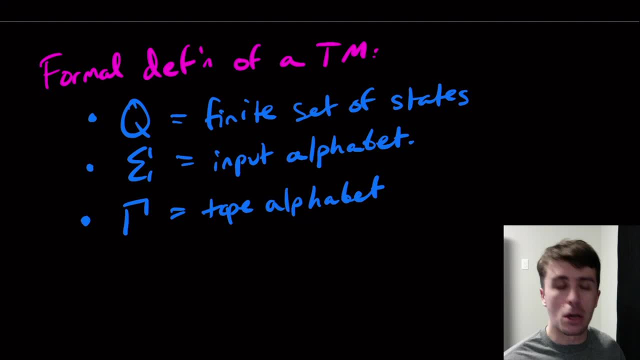 set of all things that are belonging on the tape, And one thing we can notice is that sigma is a subset of gamma. And why is that the case? Because the input is presented on the tape, So the cells of the input better be able to be put on the tape in the first place, So we can use the input as a 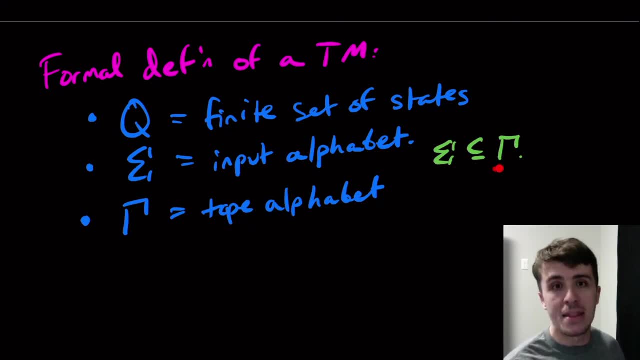 place. So all the input characters are in the tape alphabet. But one other thing we should notice is that the blank cell is in the tape alphabet, obviously because we need to acquire new cells, possibly, and we need to put blank cells on there. But we're going to say that the blank cell is not. 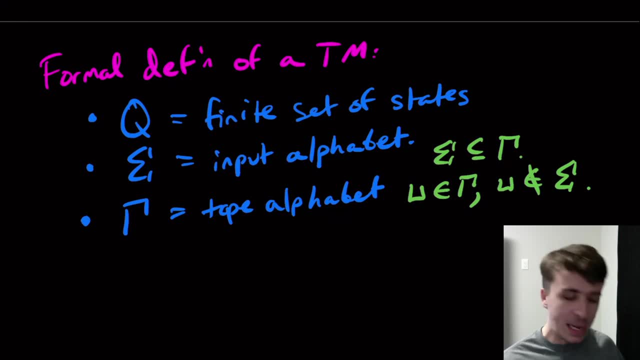 in the input alphabet. Why is that the case? Well, imagine what would happen if we had an input that had only blanks in it. So let's just say that this is the input right here, Right here. How would you know whether or not this is the empty string or an input with three? 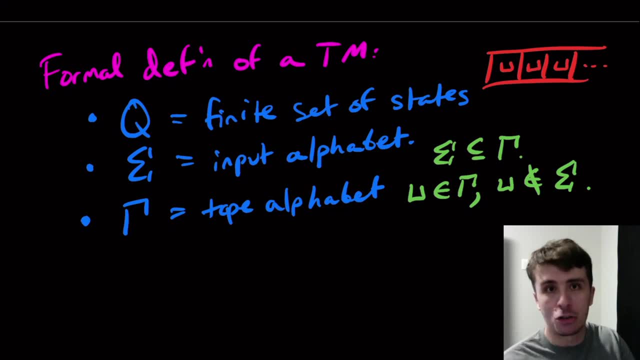 blanks in it. You don't actually know, because the blanks are all the same. So we're going to say that the blank cell is a special symbol that is only on the tape but not in the input. So if we do get something like this, we know it is the empty string at this point. 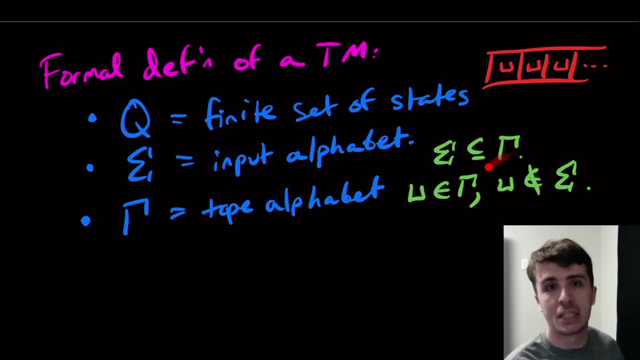 Because the first cell is a blank and the blank cell is not an input character. Okay, So what else do we have? Well, we have a start state. So this is just Q0, same as before. So this is the start. 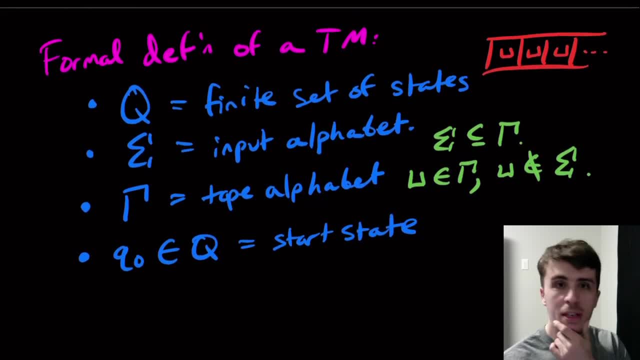 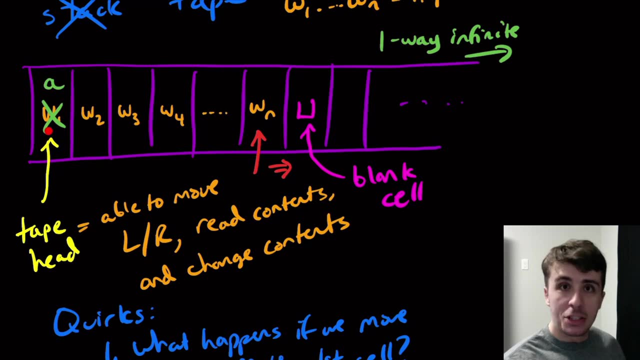 state nothing special, But one thing to keep in mind is that when we talked about DFAs just as an example, you can think of that as a Turing machine that only moves right, as I mentioned before, and once the input is done, aka we hit the first blank cell, then we can just stop at that. 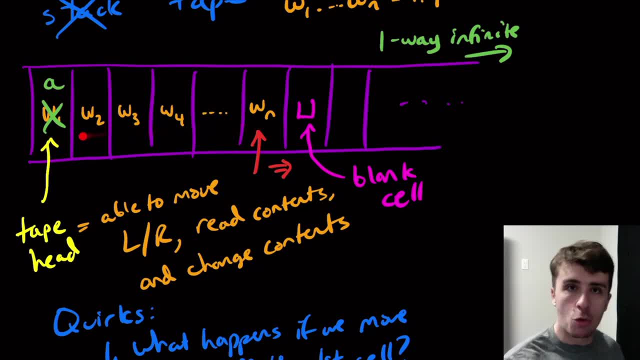 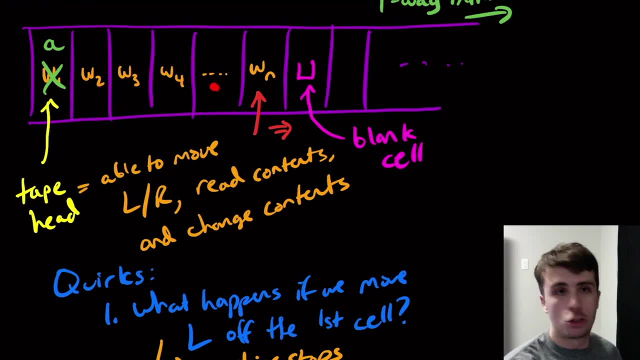 point, because the DFA is never going to go backward through the input. So if we allow the Turing machine to change cells at arbitrary points in the input, then what happens is that we don't know when we're actually done. necessarily, because it can't just be that when we go through the input we're done, because we might come back. 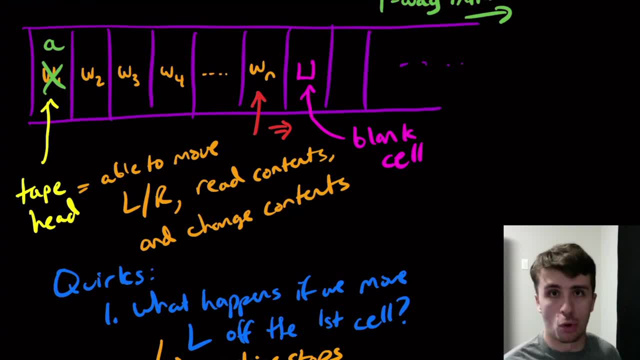 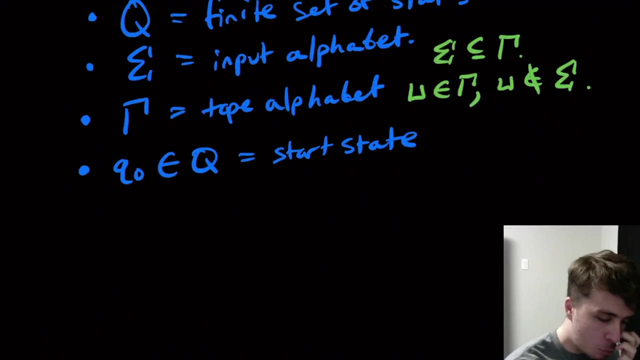 through the input and then change cells later and then do some more work. So we can't just say that a certain cell is a final state or not a final state. We need a special place to force the machine to stop, And the way to do that is we're going to have two states: QAccept and QReject. So 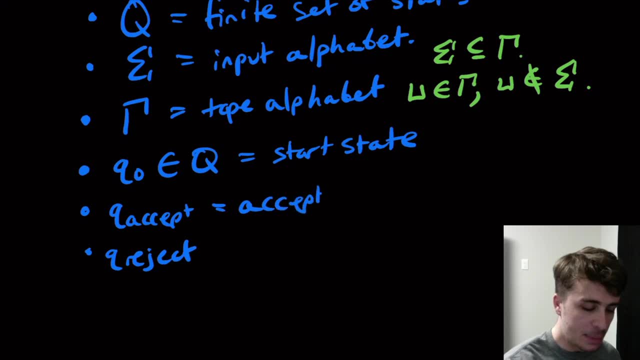 these are two special states. So this is the accepting state, So it is a special state for purposes of accepting the input and we're going to have an explicit reject state. And another reason why this is important is: at every single point, we will always have a transition to apply. 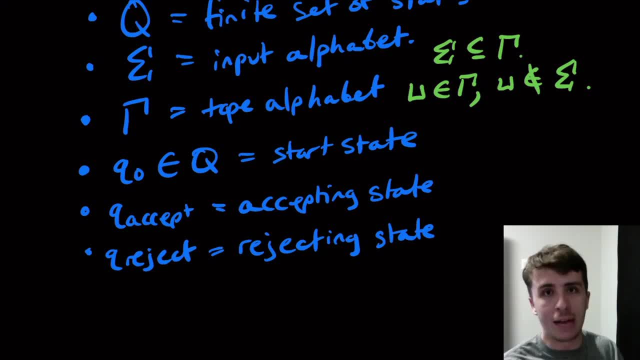 assuming we don't hit the left hand of the tape and go left or whatever. assuming we don't do that, We will always have a transition to do So, because there's always a transition to do and there's no way to classify whatever. what state is a final state or not? we need an explicit state. 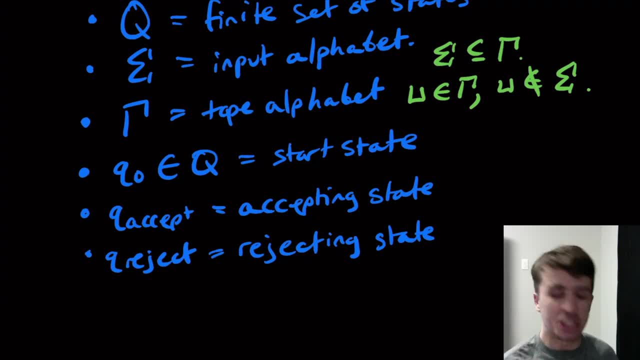 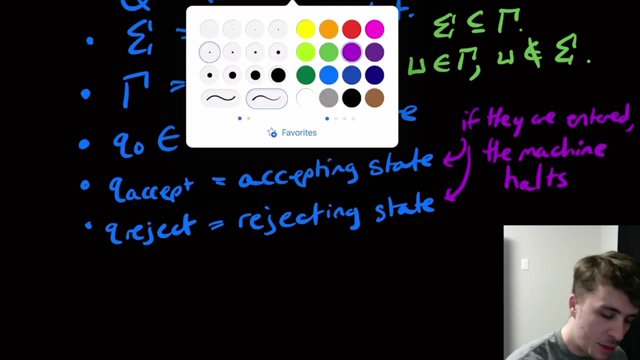 that if we enter these states then we must stop. So the behavior of these two states right here is that if they are entered, the machine halts, And so this is a special term, So halts, let me write it better- So halts. So this means either accepts, 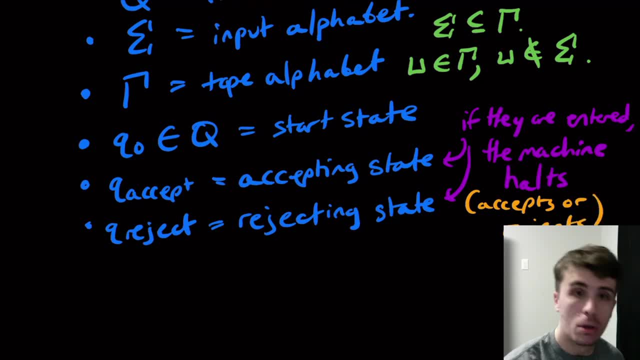 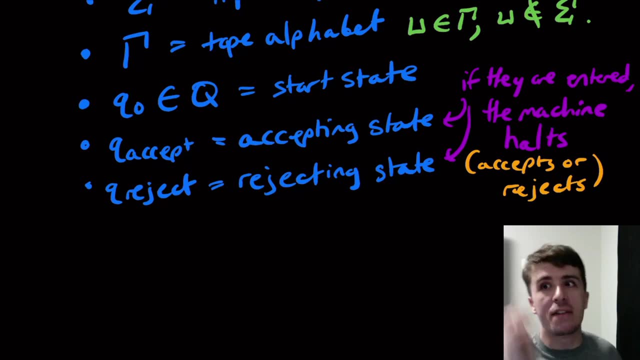 or rejects, depending on what we're doing. So whether or not we enter the accept state or the reject state means we accept or reject the input, Whereas with the DFA you just had to go to the final state after having read all the input. And same thing with the PDA. 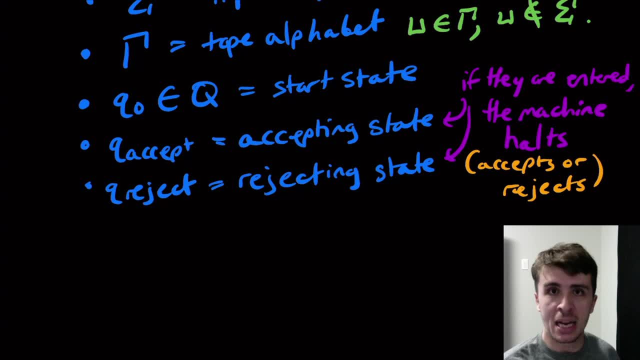 we need an explicit state to actually say we're going to stop right now and accept or reject, And Ok. and then the final piece- and I'm going to do it in red- is delta, which is the transition function. So this is the transition function. 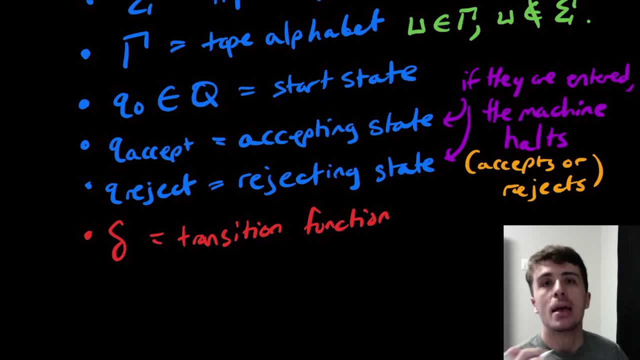 And how does it work? Well, it's a state-based machine, just like before. so we have to take a state and we need to be able to look at the cell that that the tape sendlight and end to work at head is looking at, and then decide what we need to do. So those are the only things, the pieces of. 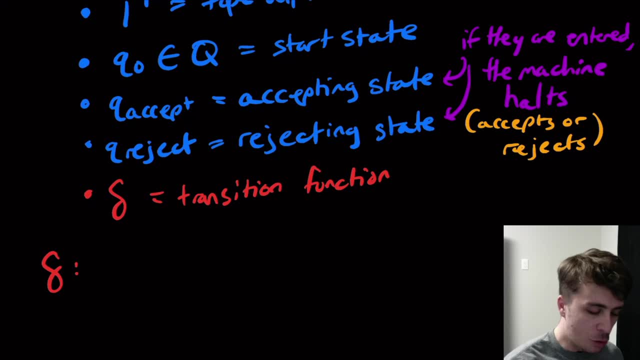 information we need to know. So delta is going to be a transition, a function from q times a gamma, because we got to take a state and a tape symbol. and it's okay because we don't have to put the input alphabet or whatever here, because we you can just define this for any tape characters that. 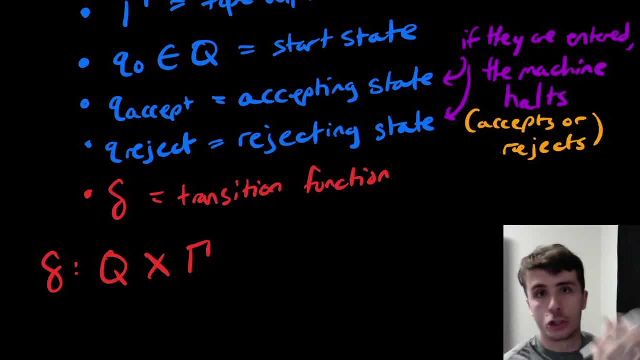 are not part of the input, because all input characters are in the tape alphabet anyway. So this is totally fine, and once we do that, we want this machine, at for now at least, to be deterministic. so we got to figure out what state to go to. so q here, and we also need to figure out what thing to 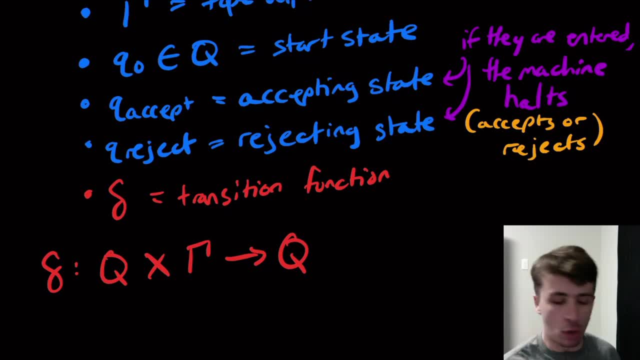 write into that cell, whatever one that we're looking at. So q cross gamma again, because so gamma on the on the right is the thing we write. actually, I should write all these. so this is the state that we are currently in. so this is the current state. so this is the observed cell content. whatever is in that. 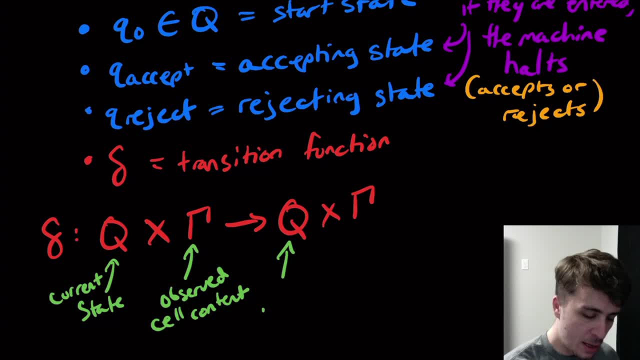 cell. this q is the next state that will be wherever we're going to. this gamma is what we are into that cell. whatever we're writing into that cell, It could be exactly the same thing, but we're always going to be writing something into the cell. It could be the same, that's. 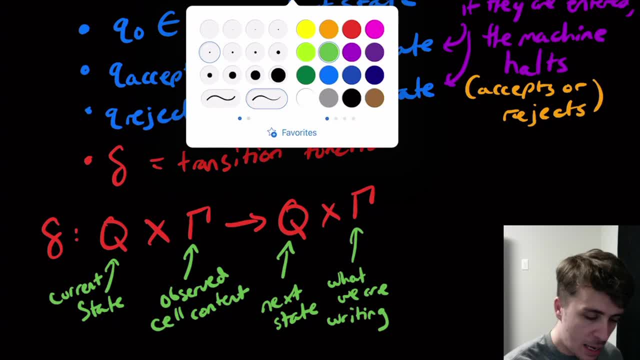 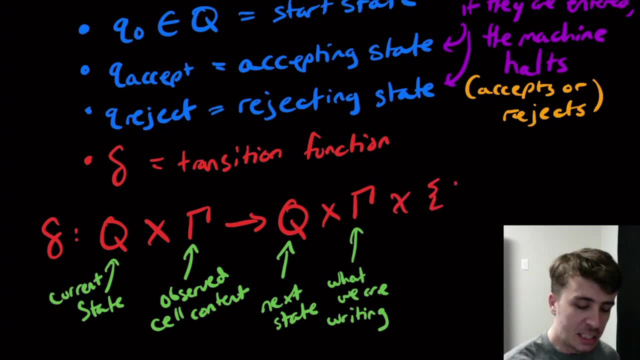 totally fine. but we're always writing something And then after that we need to figure out whether to move left or right. So I'm going to put cross the set which contains two special symbols. They're not anything on the input alphabet or the tape alphabet or whatever. It's just to specify. 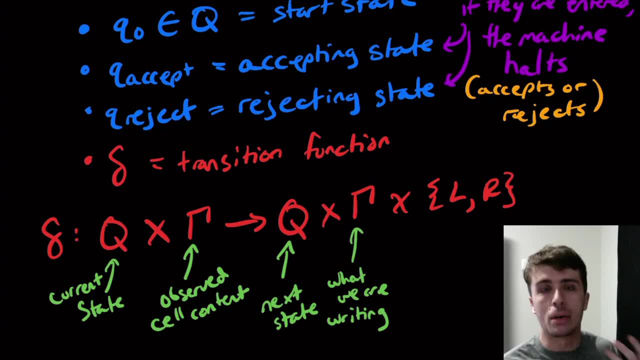 the transition function and to make the Turing machine state diagrams later. So it's just a set with two things in it and we choose. either we go left or we go right. So this will be the direction of the tape head, Okay, and whatever it moves- left or right And 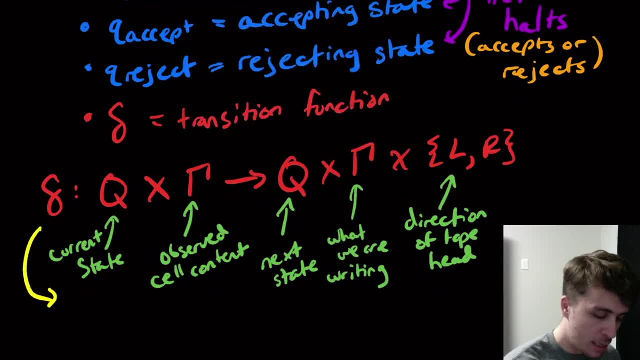 this is the direction of the tape head, And this is the direction of the tape head. And one thing that we will also note is that delta is a total function, And I mentioned this when I talked about DFA's way back when- but this just means that, no matter what state you have- and 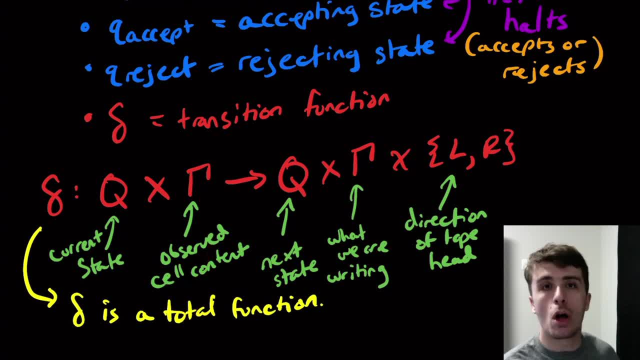 whatever style content you have, you will always have exactly one transition to do. And that is exactly the same idea as a DFA, except we have two things to worry about instead of one. Actually, no, No, we have two things, just like DFA's had. Every state has every possible input character.